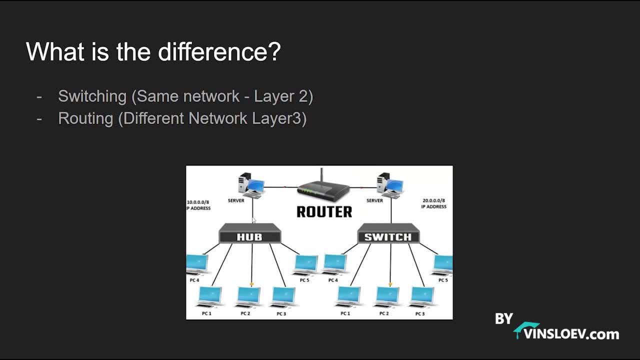 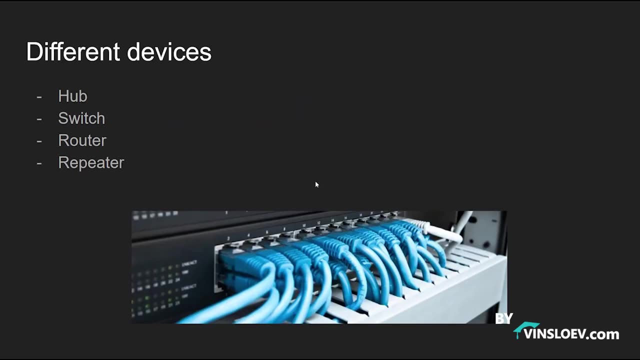 Whereas routing is communication between different networks, And that is why you see these two devices- hub and switch- is on their own network, whereas a router is connecting them. So what is the different devices that we are going to talk about? We are going to talk about a hub switch, a router and a switch. 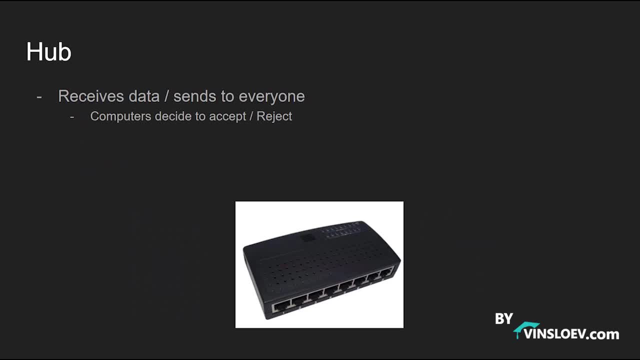 So what is a hub? Well, a hub is a very dumb device, As you see in the picture here. you have probably seen one before, or you maybe use one in your own network right now, But what a hub does is basically just receive data and then send it out to everyone connected to the hub. 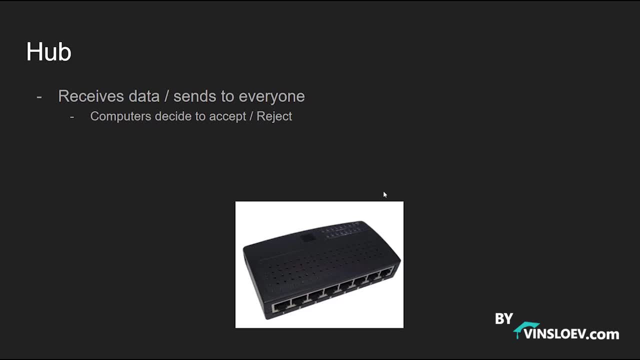 And then it is simply up to the computers to decide whether they want to accept or reject this communication. This means that if you are sending some information to user B, then if you have a malicious user on device C, then unless his computer rejects the information to user B, he will actually also get that information, because the hub doesn't care who it sends to. 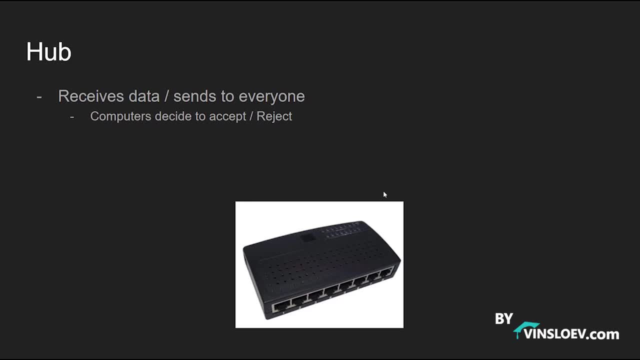 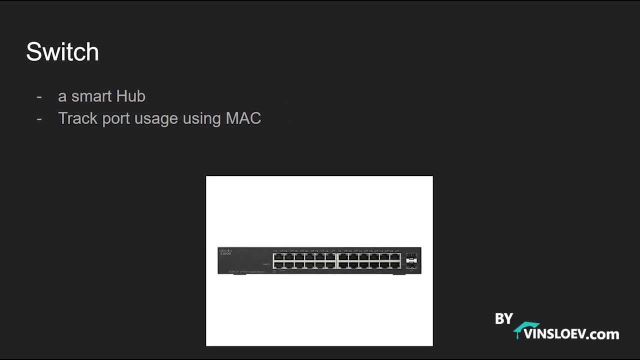 It just says, okay, here is some data, and it just pushes it out to everyone. Then we have a switch. This is This is typically called a smart hub, because it does a bit more than a hub. This one keeps track on the different computers and devices connected to it. 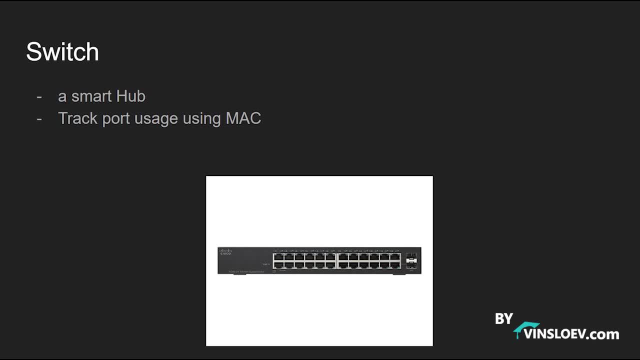 It does so by making tracks in a table of the MAC addresses. We have discussed MAC address in previous sections And this is layer 2 in the OSI model. So the switch will start to record what kind of MAC address is being used from the different port within the device. 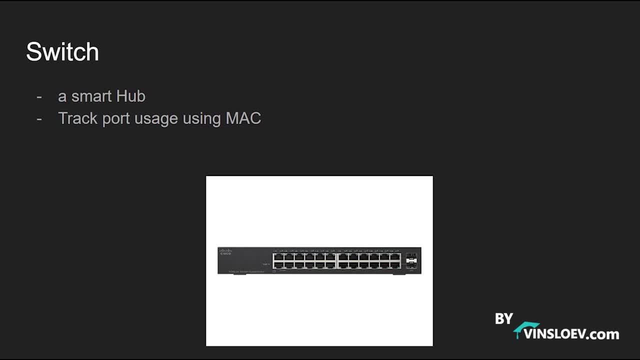 And then it will keep track on what port a specific MAC address is connected to, Because then it knows that if some information comes from this MAC address to this MAC address, then it needs to go to these two ports. But this will happen over time. 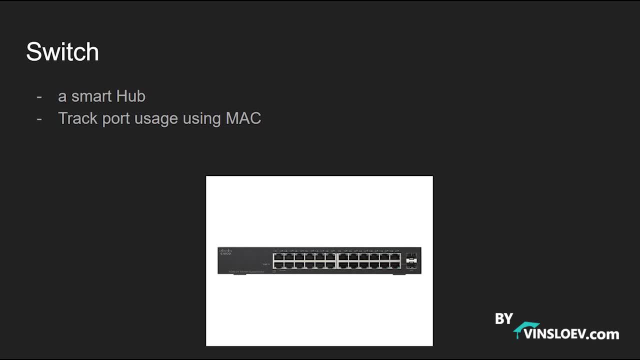 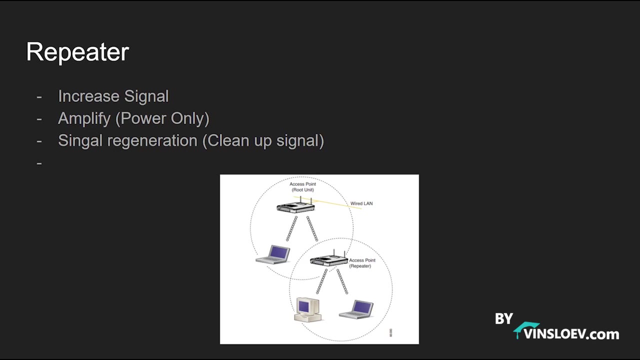 So at the beginning of using a switch, when you connect your devices, it is simply just acting like a hub until it starts to figure out which MAC addresses belong to which ports. Then we have a repeat. A repeat is compared to switches and hubs. 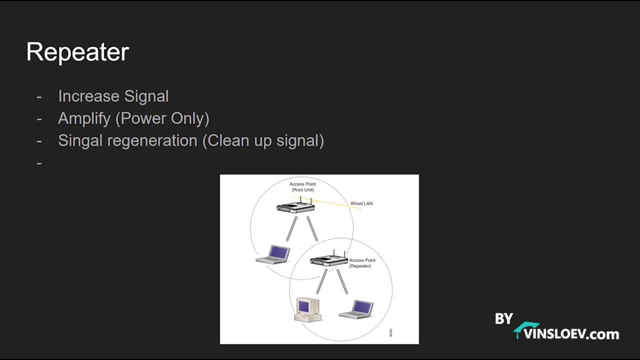 It is used for making the signal stronger And, as you see on the picture right here, we have a repeater at the end of the range of this wireless network. And because we have this repeater, then it is capable of receiving messages from this computer right here. 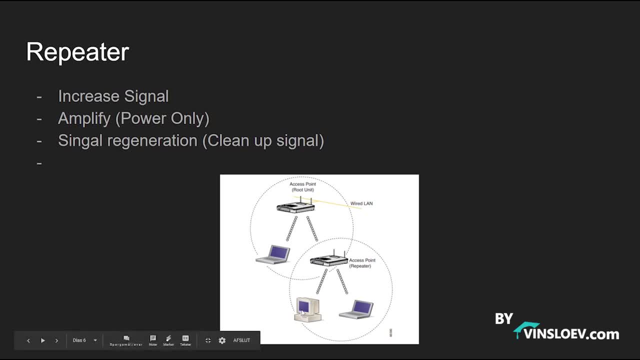 And then enhance the signal So that it can reach the computers. that is actually without the range of this main point right here. And it can do so in two different ways. It can amplify, meaning that it just smacks the message out with more power. 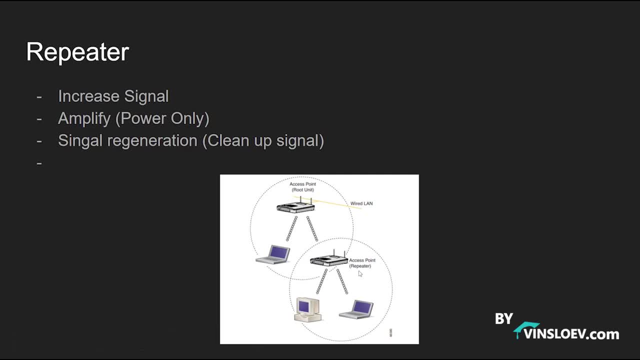 And it can do signal regeneration, meaning that it tries to clean up the signal, Because when a message transfers, either through the air or through cable, there will be some magnetic interference- electric magnetic interference- that will, at the end, destroy the package, And that is why we have these ranges. 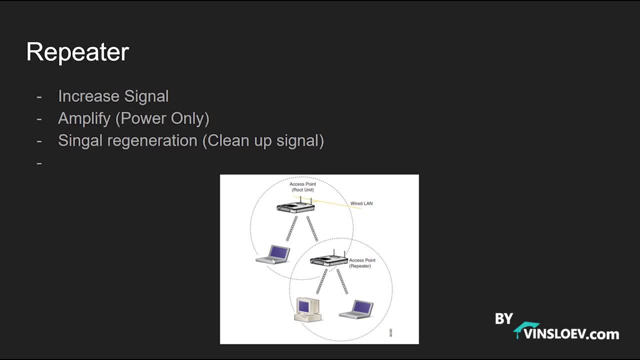 Because at some point the device is simply not able to reach out anymore. So by having this repeater it can enhance the signal so that we can reach a much larger area. So you can set these repeaters up on your network At specific locations where you want the signal to be enhanced. 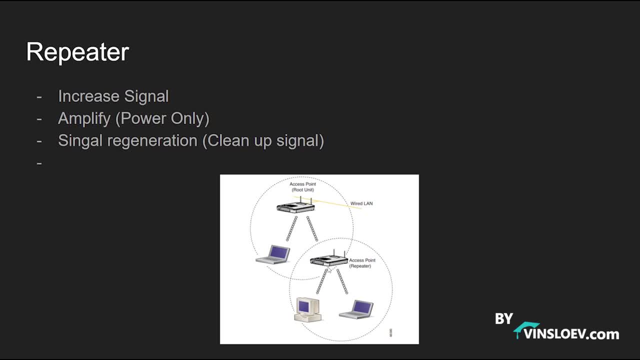 This can be where you have thick walls Or where you simply just have a too long of a path between your devices and your main router, For example, if you have your router located at one end of the house And you want a signal at the very end of your ground, maybe in the garage or something. 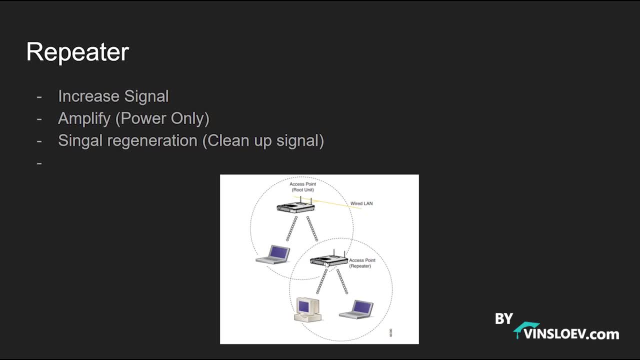 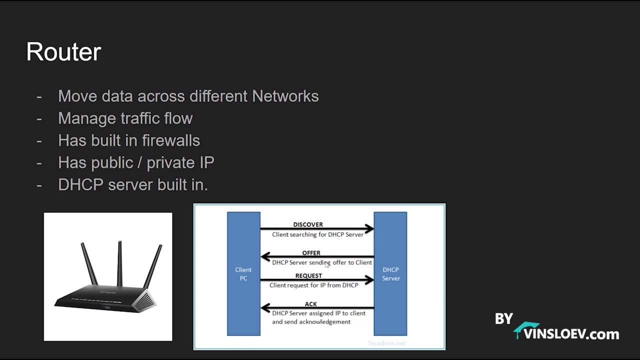 Then you can use such a repeater And at the ending we have the routers. These are the real smart devices and the ones that make all this networking possible, Because what a router is compared to a switch and a hub is a very, very smart device. 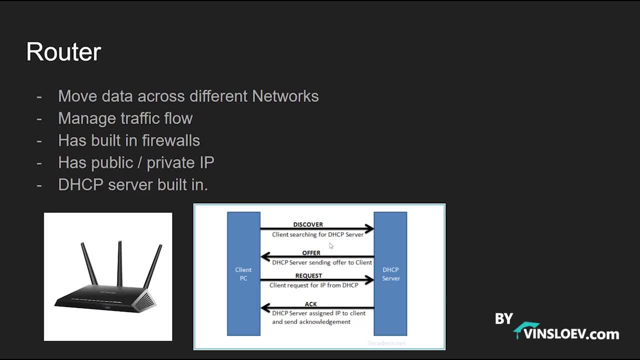 It manages all the traffic between our internal and the public network. So a router actually has two IPs. It has the public IP, which is the IP that the internet is seeing, And then it has a private IP, which is the IP used by your devices on your internal network. 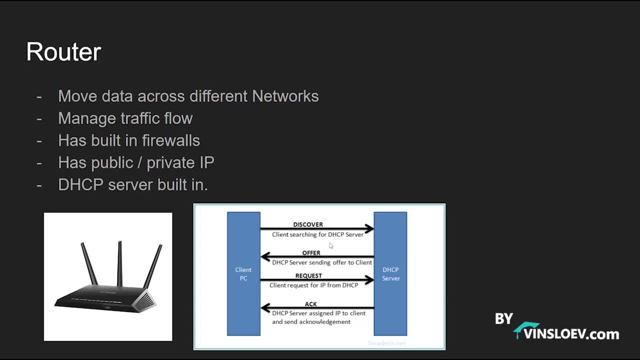 And most routers also have built-in firewalls. This means that you can manage your firewall rules based on who is allowed to connect and move the packages to and from your network and the public, Whereas switches and hubs simply doesn't have that. It will just allow everything to happen. 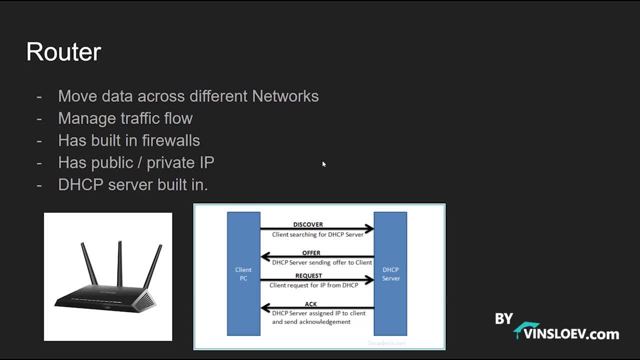 And then most routers also have what is called a DHCP server built-in, And what such server is doing is to make your computers have IPs, Because once you connect to a network- as we discussed in previous lectures about IPs and MAC addresses- Your computer will only have a MAC address. 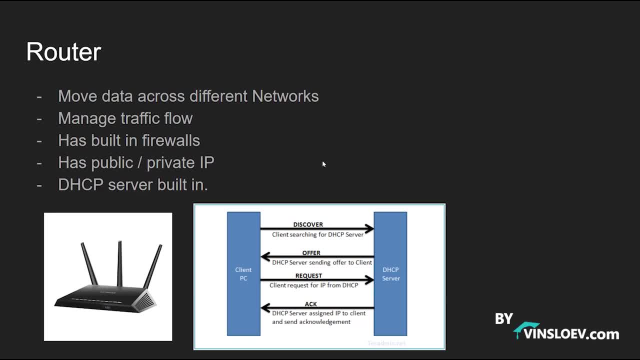 So it needs an IP From somewhere, And that somewhere is typically from such DHCP server Which is built-in to your router. So what your computer will be doing when it is connected to the network, It will use this flow right here, where we first discover. 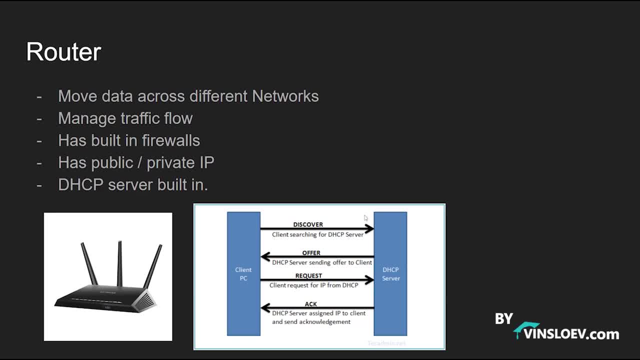 We try to find where the server is located, Then this is located probably within your router, And then your router sees this and says: okay, you need a new IP. Then it will make an offer: Use this IP, Because this IP is currently free. 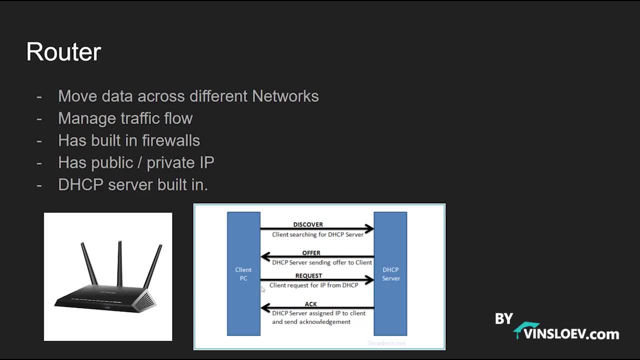 And then you will just make a request to your computer on this And say, okay, fine, I can use this IP. And then your router, which has this DHCP server, Will acknowledge and say, okay, fine, I will note that down And you are now assigned to this IP.